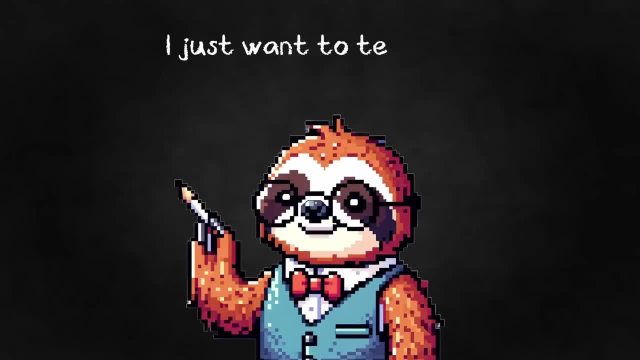 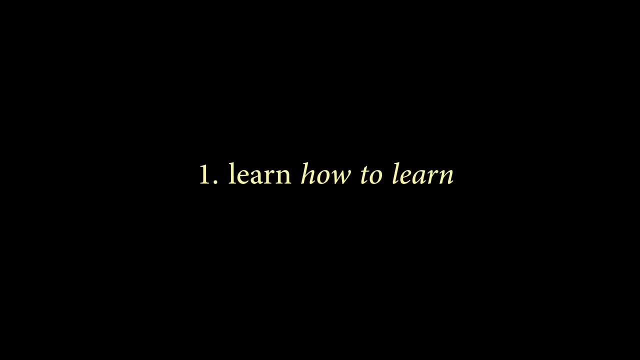 won the lottery. That does not mean it's going to happen to everybody. I'm just here to give you everything you need to get started, and I hope you understand that. So, with that out of the way, let's get started. Number one: learn how to learn. Now I know what you're thinking, Sloth. I'm here. 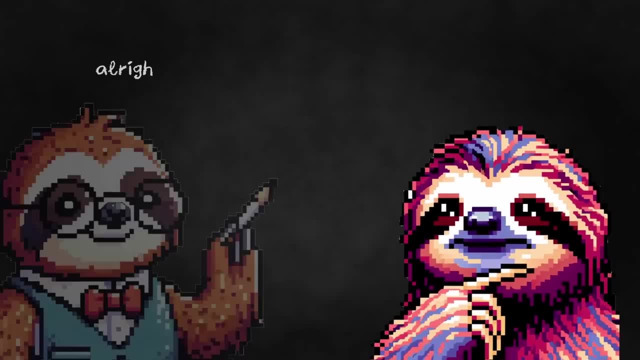 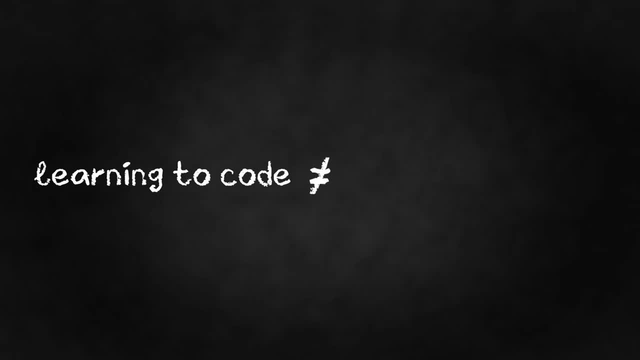 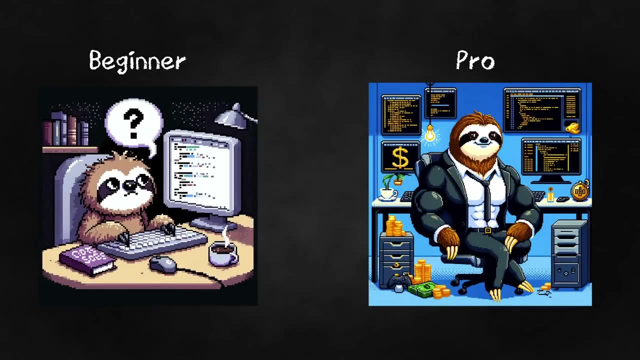 is really important. I swear this will help a lot. Learning to code is not about programming languages. It's about developing a mindset for problem solving and continuous learning. This is what separates the beginners from the professionals. The professionals know how to solve their own. 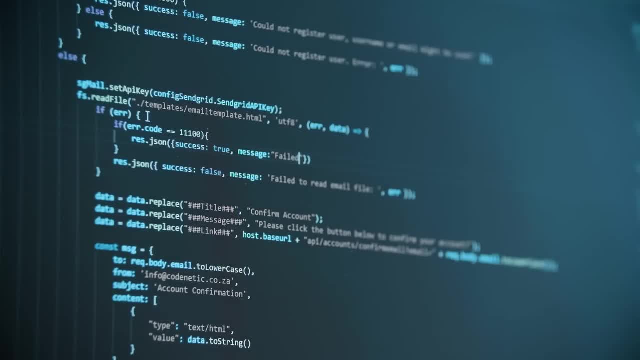 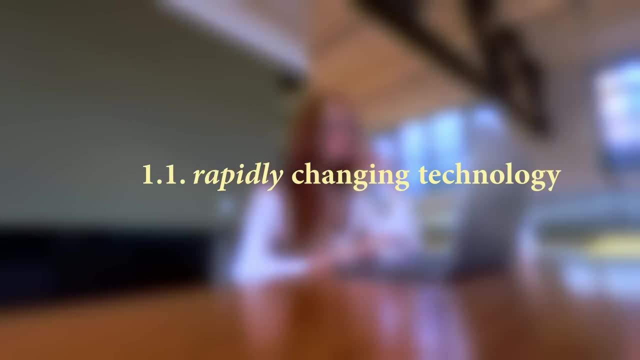 problems and learn new concepts pretty quickly, So it's crucial that you understand how to learn. But, Sloth, is it really that important, especially for coding? Yes, it is. Let me explain why. Number one: rapidly changing technology. The tech world is always evolving. New languages, tools, frameworks- they're popping up all the 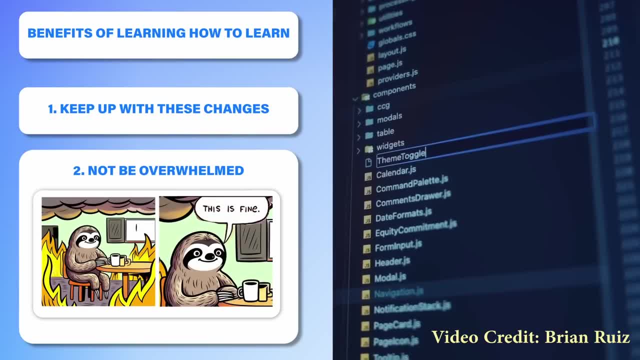 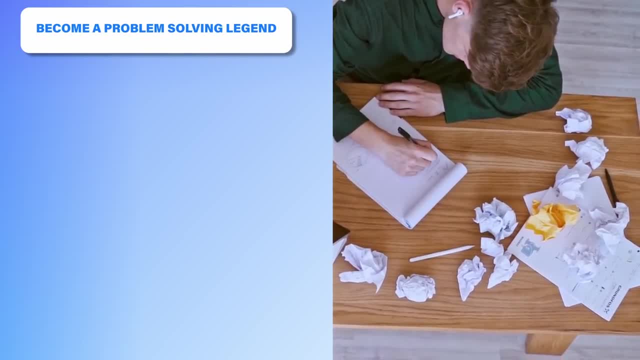 time. If you know how to learn effectively, you can keep up with these changes without getting overwhelmed. Two problem solving skills. Coding is basically problem solving. Each line of code is a solution to a mini puzzle. Learning how to learn enhances your ability to break down. 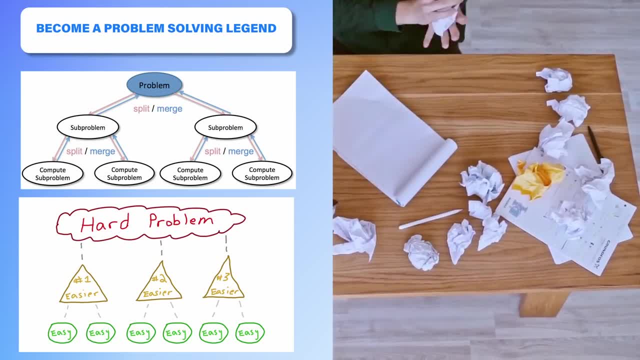 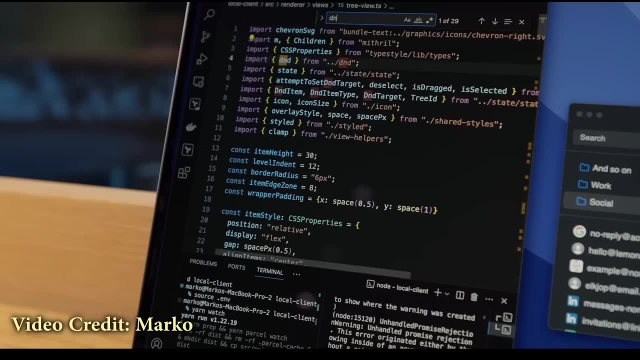 complex problems into manageable pieces and find innovative solutions. Three: adaptability. This skill is gold in the coding world. When you're comfortable with learning, you adapt better to new challenges. You're more willing to step out of your comfort zone and tackle unfamiliar tasks. Four: independent learning. You won't always have someone to hold. 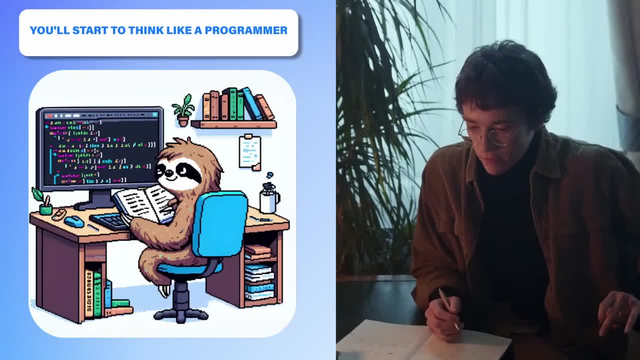 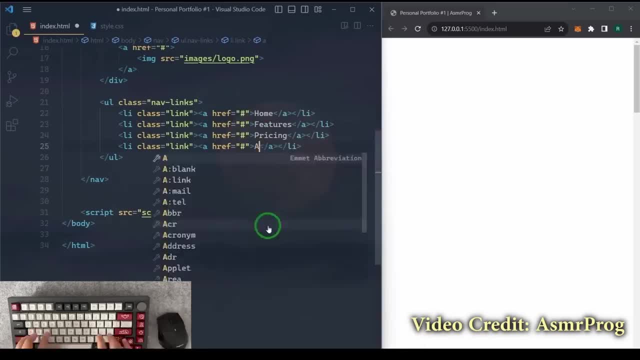 your hand through every coding challenge. Being a self-sufficient learner empowers you to find solutions on your own, making you a more competent and confident coder. Five: efficient learning Time is precious right. You want to learn to code as fast as possible. Well, by learning how to learn. 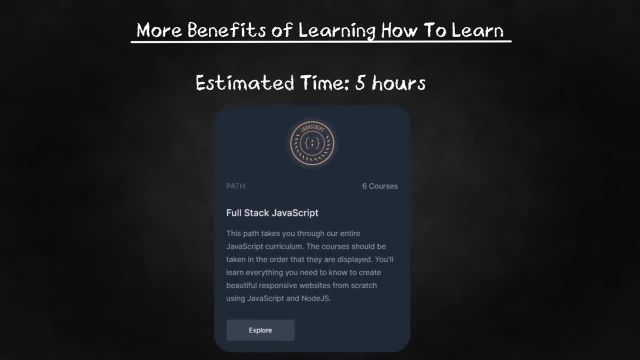 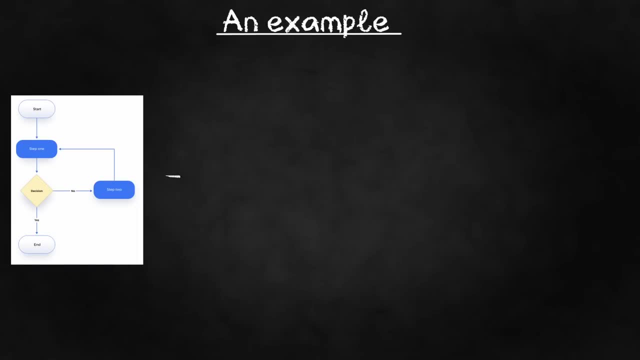 you can tailor your coding education to be more effective, where, instead of taking five hours learning a concept, you'd only need to spend an hour. Here's some examples to give you an idea. You can use diagrams to plan a simple coding project, then jump in and start building it. 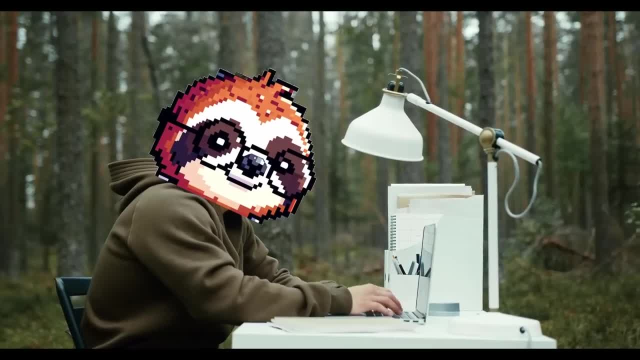 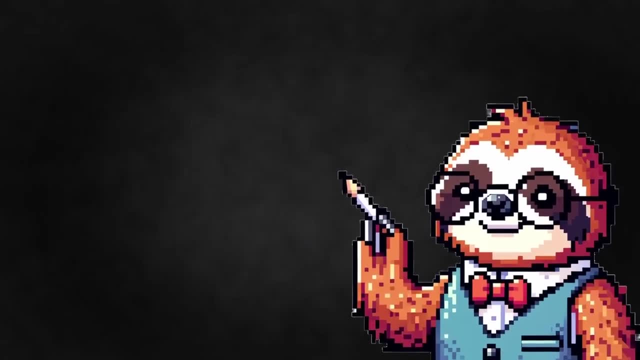 And, finally, ask people for tips on how to improve it. The key is to discover what works best for you and use it to make your learning as smooth and enjoyable as possible. Remember, there's no one size fits all in learning, especially in something as diverse as coding. While I can't directly help, 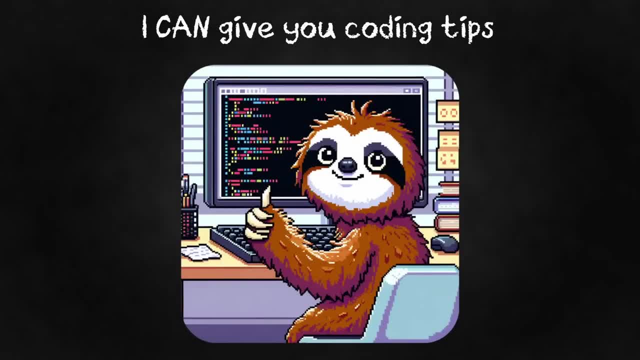 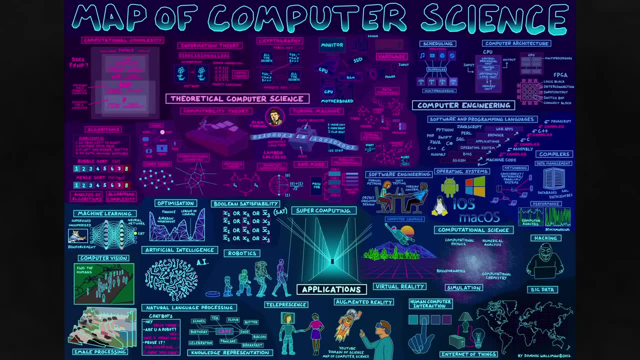 you find your unique learning style. I can definitely guide you with general tips throughout the video to speed up your progress in coding. And now for the big question: where do I start? Coding is a vast jungle, but don't worry, I'll give you a map to guide you on the right path. 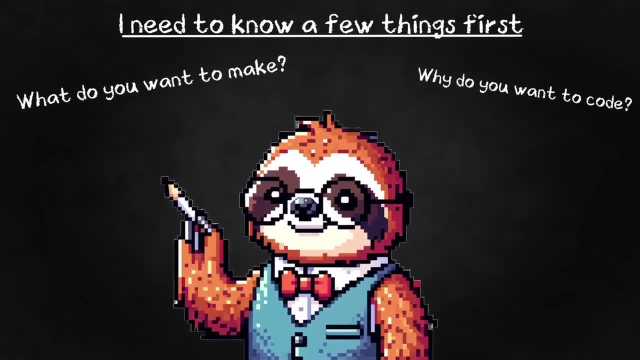 But I need to know a few things from you first. What do you want to make? Why do you want to code? Do you want a big tech job? Do you have an app idea? Do you want to make a video game? Okay, that might have been too fast, Let's slow. 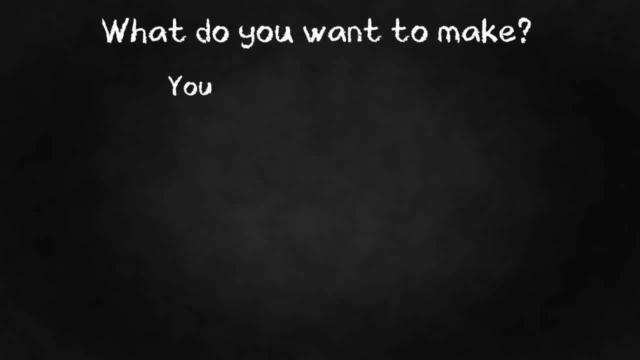 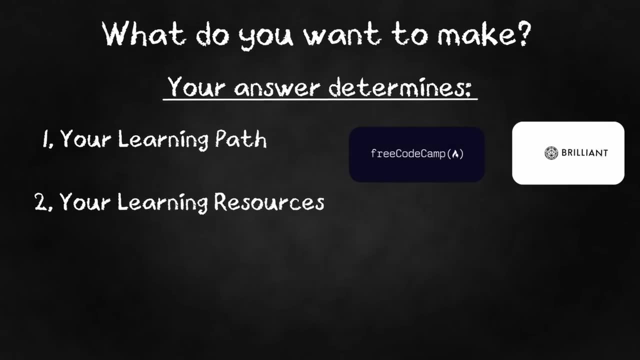 it down and start with two questions: What do you want to make? Your answer to this question will guide your learning path to make sure you're not learning something you're not supposed to and end up wasting time. It'll decide the resources you choose and the projects you'll embark on. Remember: 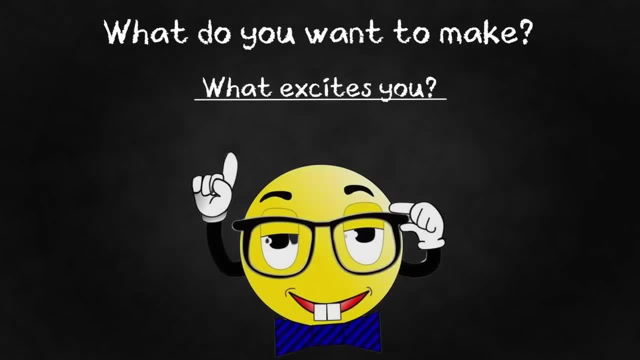 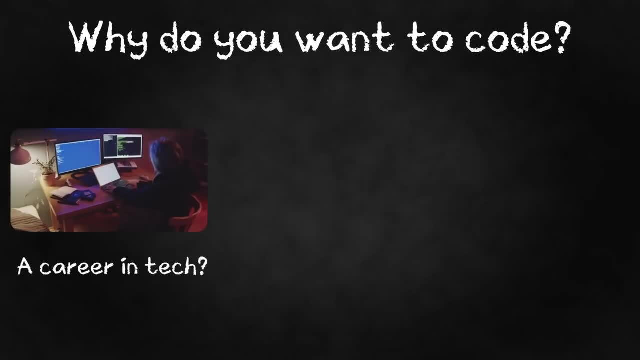 there's no right or wrong answer here. It's all about what excites you and what keeps you up at night thinking. I can't wait to create that. Now for the second question: why do you want to code? Are you looking for a career in programming? 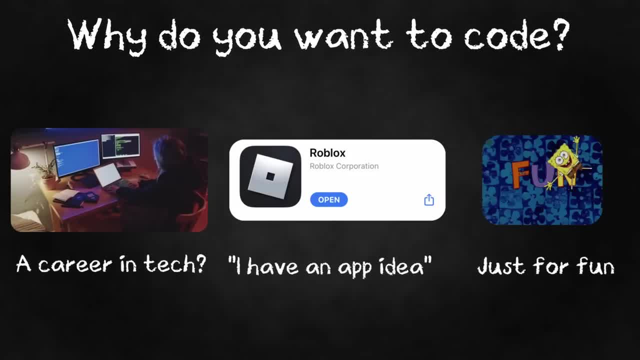 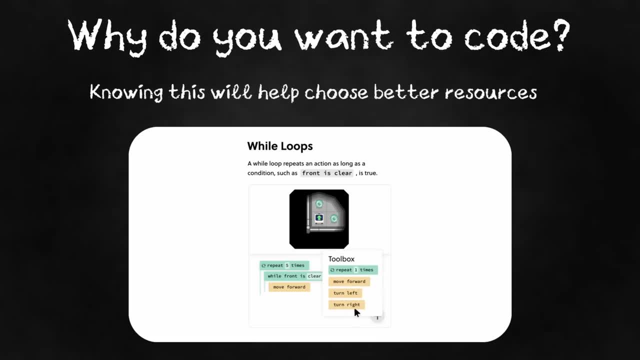 Do you want to bring a unique app idea to life Or are you just coding for fun? This is what's going to motivate you when you eventually hit that bug at 2am and can't figure out why your code isn't working. Understanding your why also helps in choosing the right resources If you're 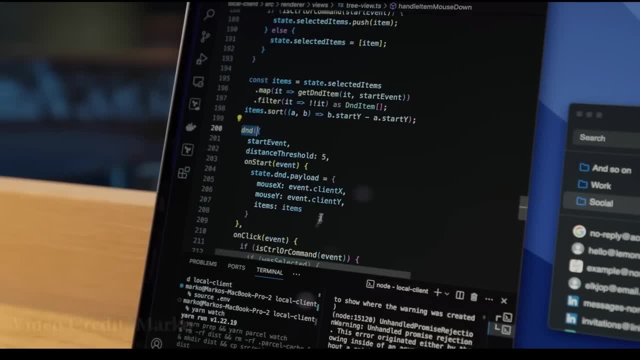 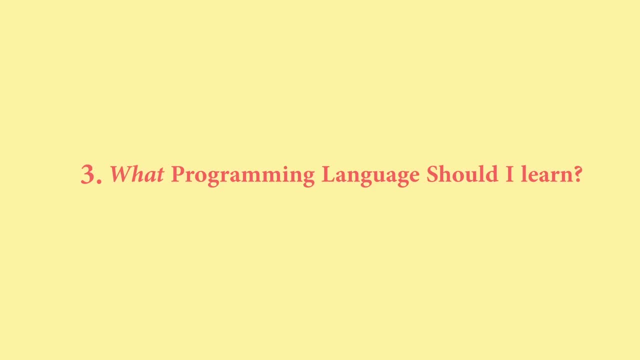 career focused, you might lean towards areas that are easier to get a job in. If it's a hobby, you have more freedom to explore certain areas. Now that we've got your what and why, let's talk about the how. Three. what programming language should I learn The programming language? 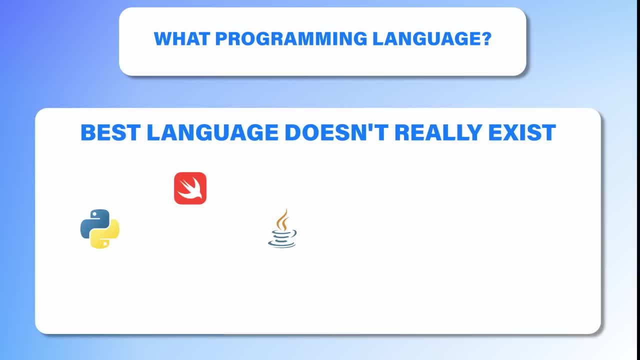 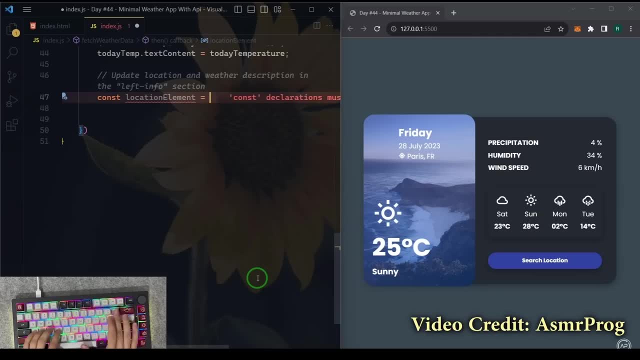 you should learn all depends on your answer for those two questions. There's no such thing as a language, but there does exist popular languages. Let me explain what you should research based on your interests. If you want to build websites or web applications, start with HTML CSS. 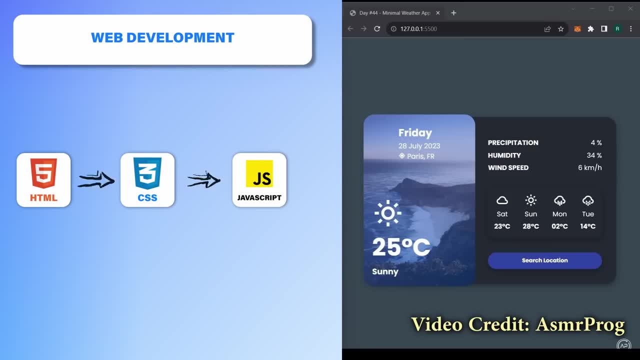 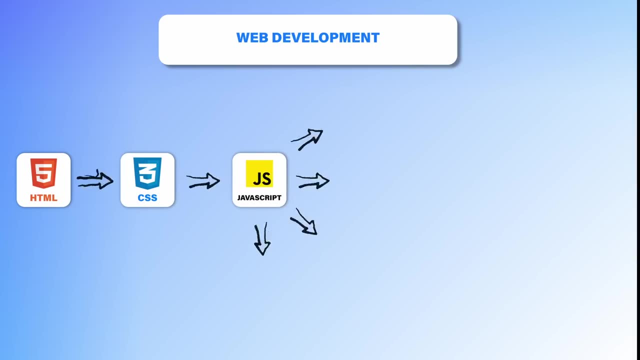 and JavaScript. These are the main technologies of the web. HTML structures your content, CSS styles it, and JavaScript adds interactivity As you advance. consider learning frameworks like React, Vue, Svelte or Angular for more dynamic and responsive applications From there. 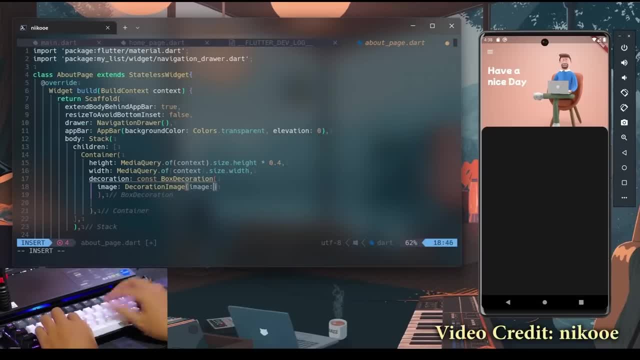 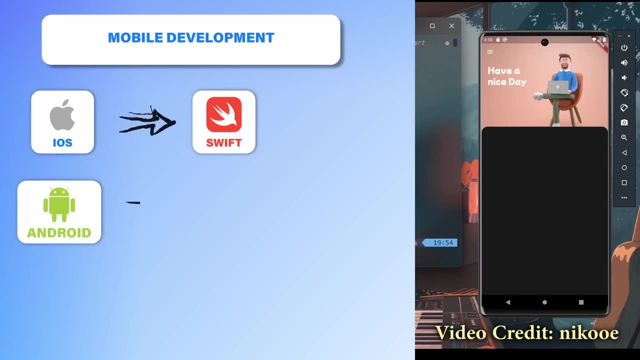 you can start learning some backend. If you want to build mobile apps, your path depends on the platform For iOS apps. learn Swift. It's Apple's modern programming language for iOS. For Android, start with Java or Kotlin. Kotlin is the newer language and it offers more. 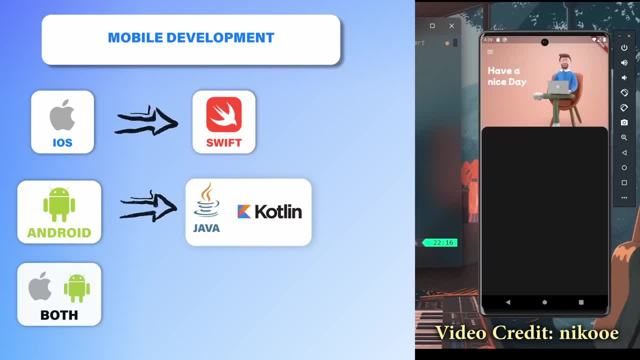 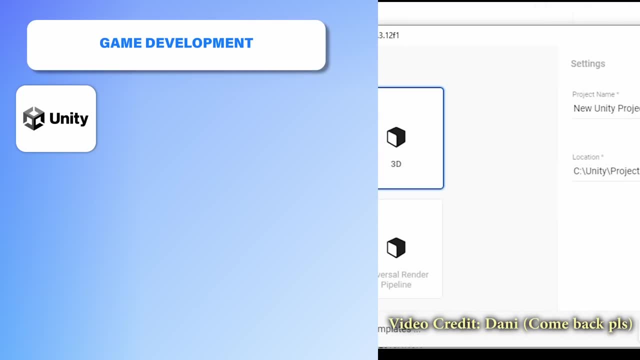 modern features and is now preferred by Google for Android development. If you'd like to do both, consider learning, React Native or Flutter. For those of you who want to build video games, check out some video game engines like Unity, Godot and Unreal Engine. Unity and Godot uses 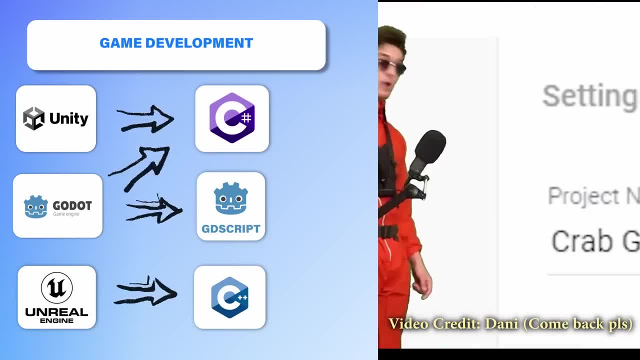 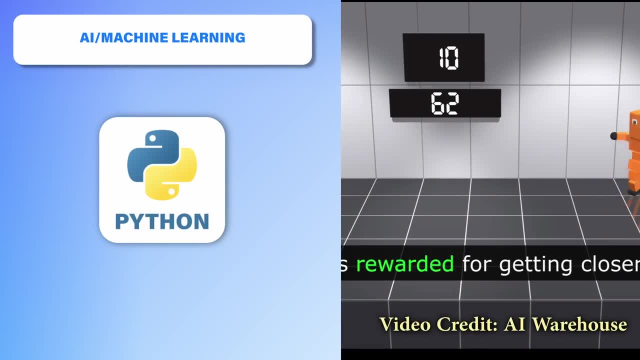 C, Sharp and Godot has its own language, while Unreal Engine primarily uses C++ And for those with AI and machine learning, Python is your starting point. This area is not just about coding. Be prepared to learn a lot about math, especially statistics, calculus and algebra. 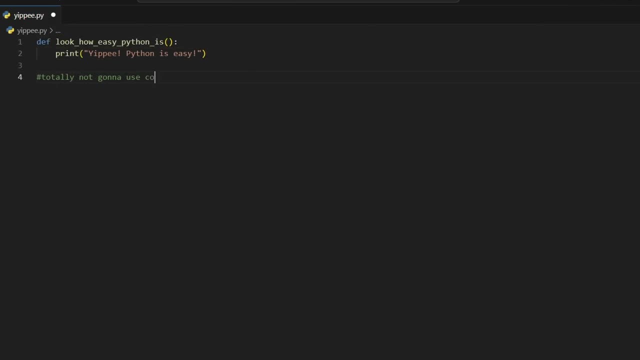 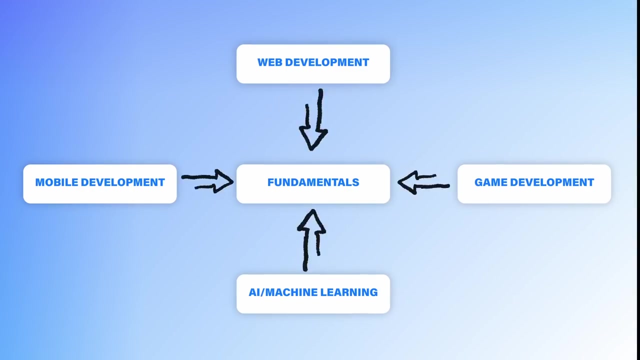 Python is the most common language in this field for its simplicity and the powerful libraries like TensorFlow, PyTorch, Psychic, Learn and a lot of other libraries that support machine learning operations. In each of these paths, your foundation is crucial. Once you grasp the basics, you can 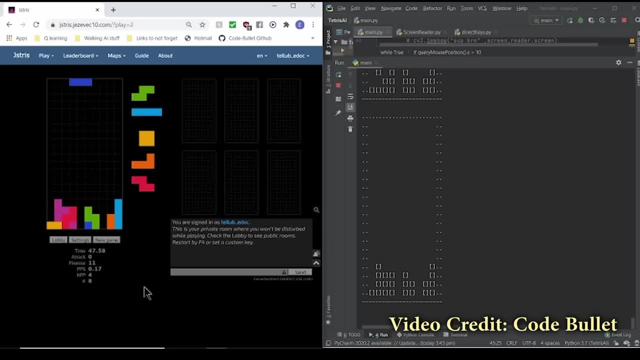 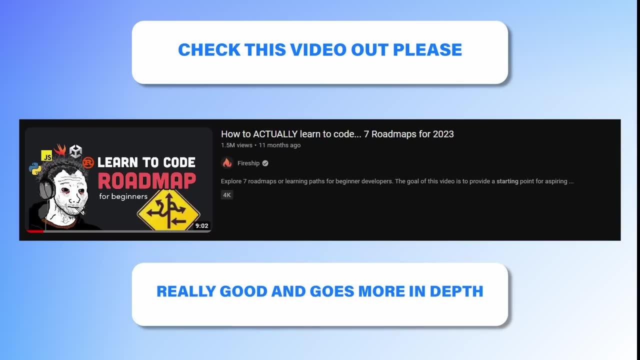 delve into more complex projects and refine your skills in your chosen area of interest. There's a lot to learn about coding, so I strongly suggest you check out this video here if you want a high level roadmap of every main area of programming to get you started Now that you have an idea of 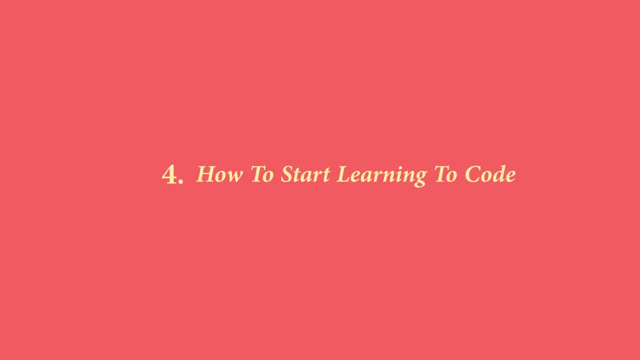 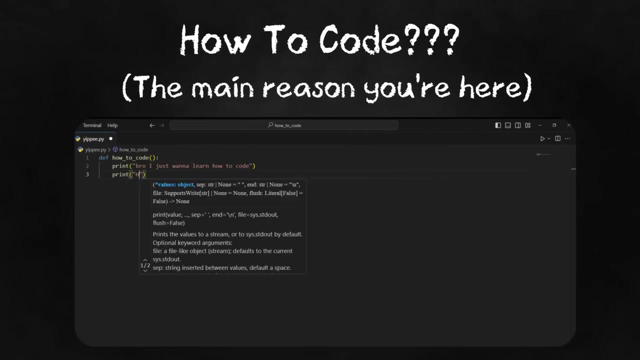 what programming language to learn. we can move on. 4. How to start learning to code. So far, we've discussed picking the right programming language and understanding your why, but what about the actual learning process? You know how to code. First off, let's talk about resources. 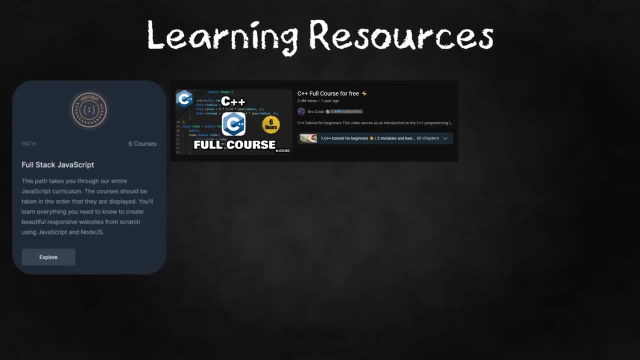 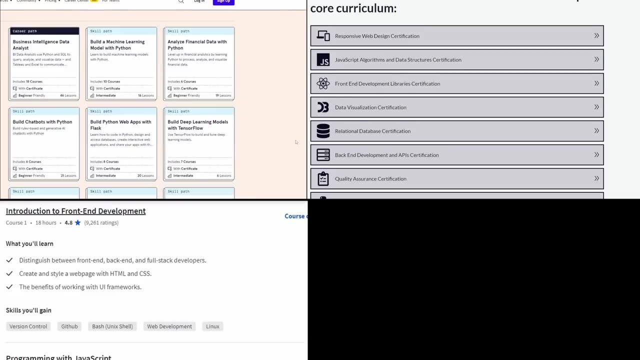 There's a wealth of information out there from online courses, YouTube videos, books, tutorials and coding communities. There's websites like Code Academy, FreeCodeCamp, The Odin Project and Coursera. They offer structured courses that are great for beginners. YouTube definitely has its fair share of tutorials, but also don't overlook the 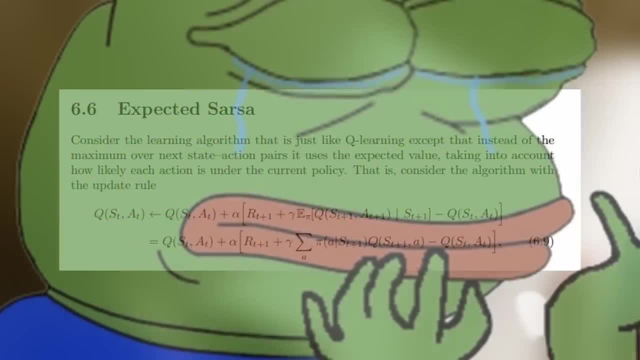 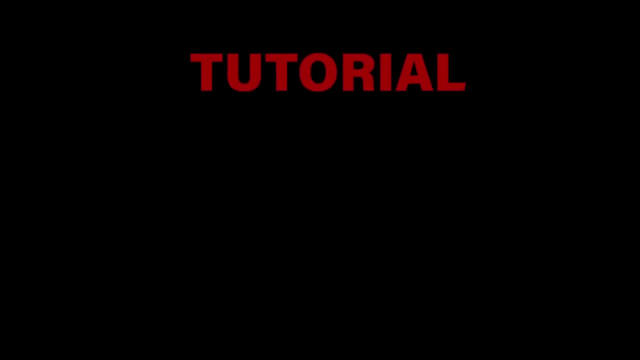 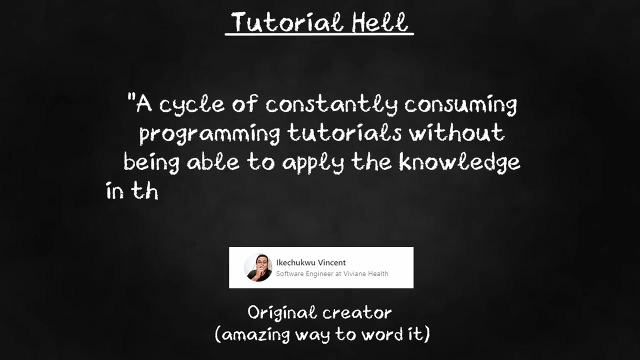 power of books. They often go deeper into concepts than many online resources. However, there's a common pitfall that almost every beginner gets stuck in: that you should watch out for Tutorial Hell, A cycle of constantly consuming programming tutorials without being able to. 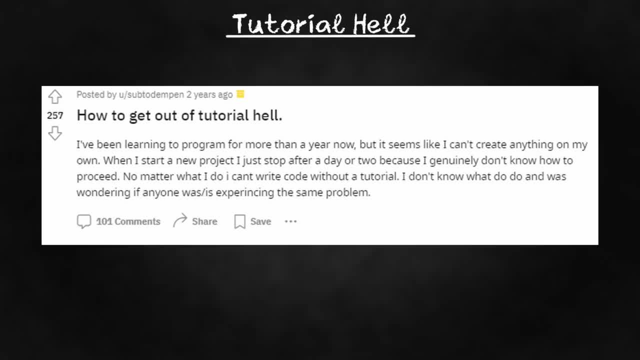 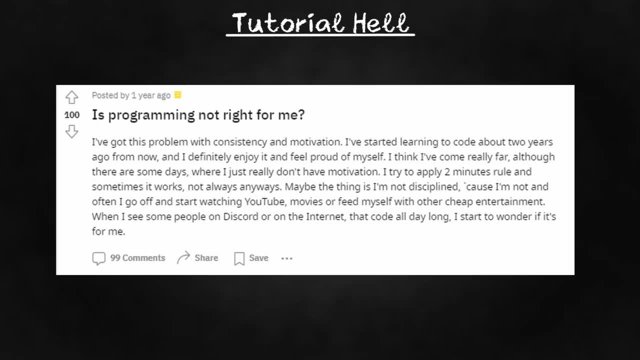 apply the knowledge in the real world and build real apps. Tutorial Hell is one of the worst things to ever get stuck in. You feel like you're not growing or improving, where, if you stay there, you'll want to quit because you feel like this is not for you. 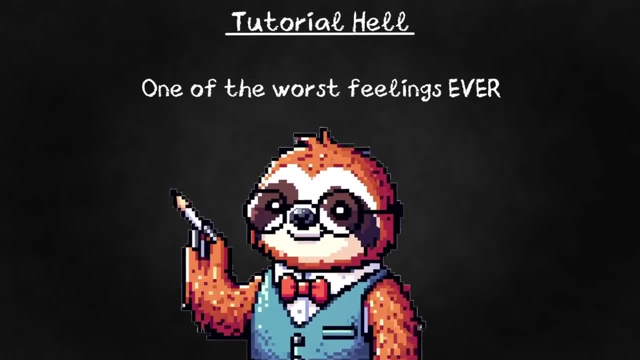 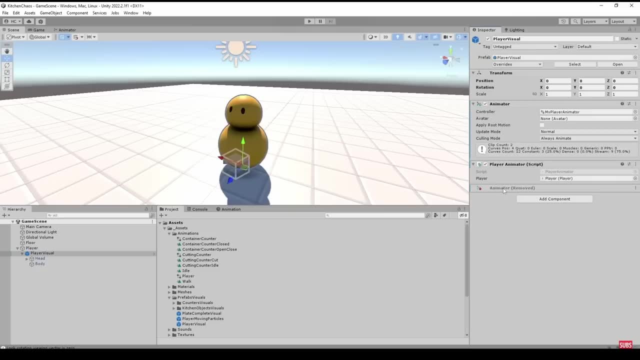 I was stuck at Tutorial Hell at one point and it was one of the worst feelings ever. I really wanted to quit programming because I felt like this was not for me at all. I kept watching tutorial after tutorial and I just felt like I never got better. for some reason, It's easy to get stuck in a loop. 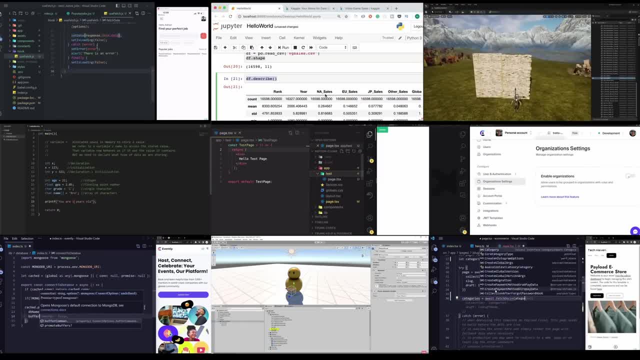 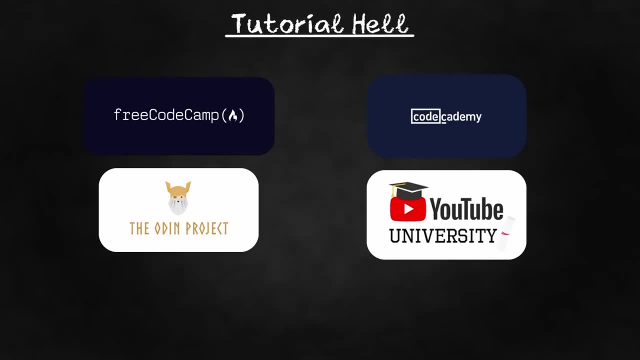 of constantly watching tutorials and courses without really applying what you've learned. While these resources build your foundation, they don't always push you to the next level of solving real-world problems. This is where the learning resources you pick make all the difference. If you do prefer tutorials, one of the best. 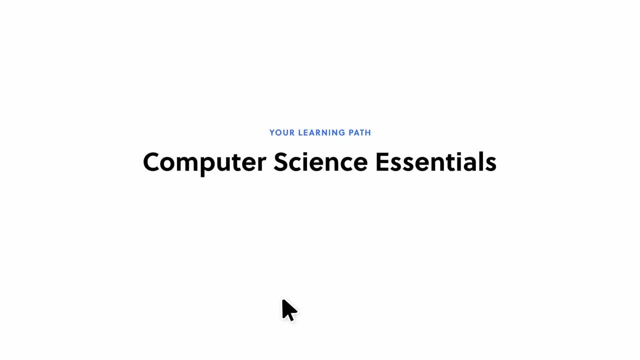 resources out, there is today's sponsor, Brilliant. Brilliant sets the standard for interactive learning for computer science, data science and math. Brilliant stands out from other learning resources because it focuses on active problem solving and interactive learning, which will help you get out of Tutorial Hell, Since learning is not about watching and repeating, it's about 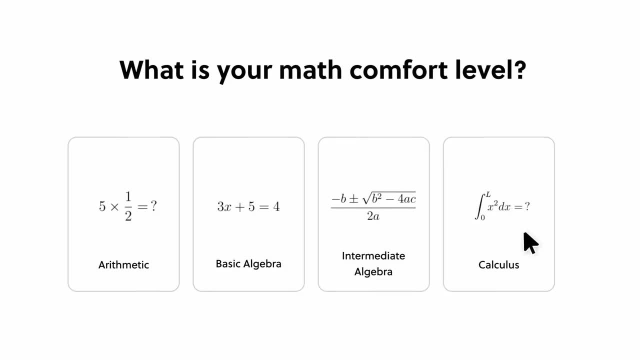 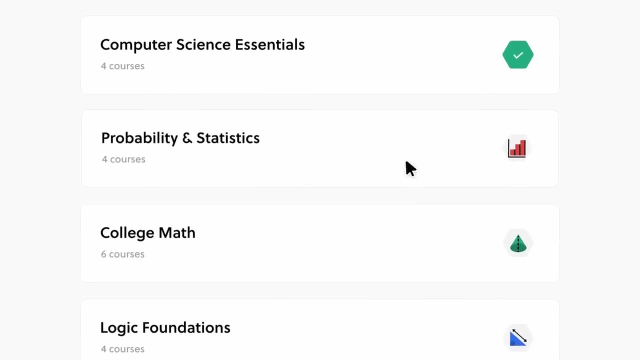 challenging yourself, and Brilliant does exactly that By customizing the content to your skill level to make sure you're learning at a comfortable pace. they offer thousands of lessons, from basic topics such as loops and conditionals to advanced topics like AI and neural networks. You'll never 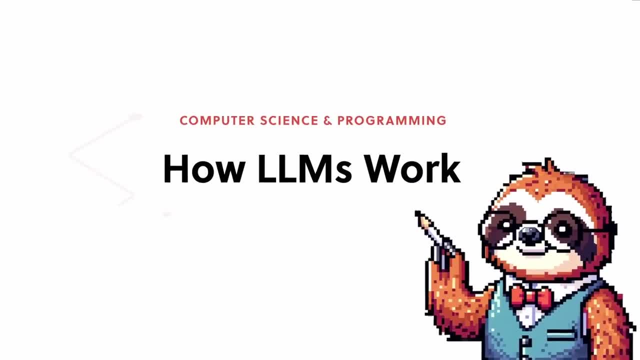 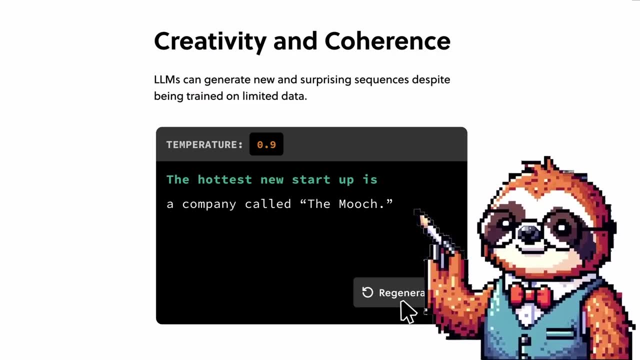 get bored, since new lessons are added every month. One of my favorite courses that they recently added is How LLMs Work, where you get to learn how something like ChatGPT works. They explore topics like how do they predict the next word and how they're so creative And the best thing about it. 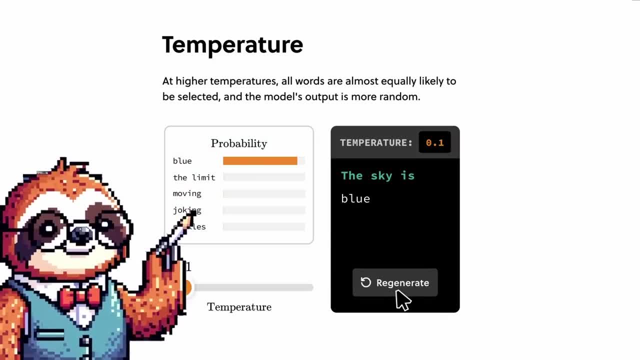 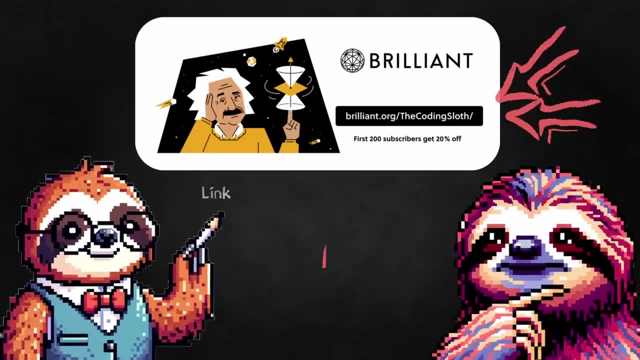 is. I learn and remember the concepts better because of how interactive it is. So if you'd like to try everything Brilliant has to offer for free for 30 days, visit brilliantcom or click the link in the description. The first 200 of you who sign up will get 20%. 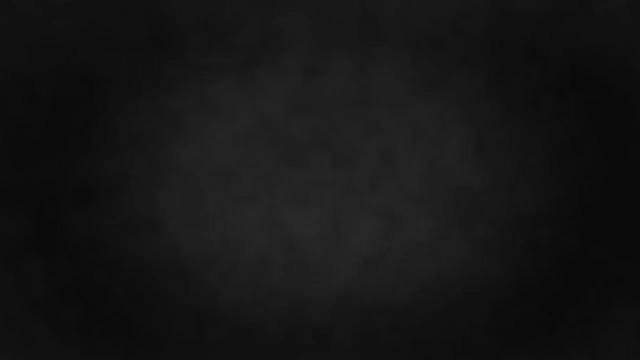 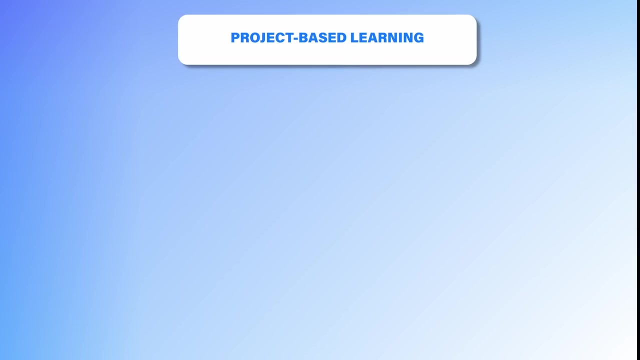 off Brilliant's annual premium subscription. You're welcome. Enjoy it Now. if you prefer something other than tutorials, then the key to breaking out of Tutorial Hell is to start practicing project-based learning. This means applying what you've learned to real-world. 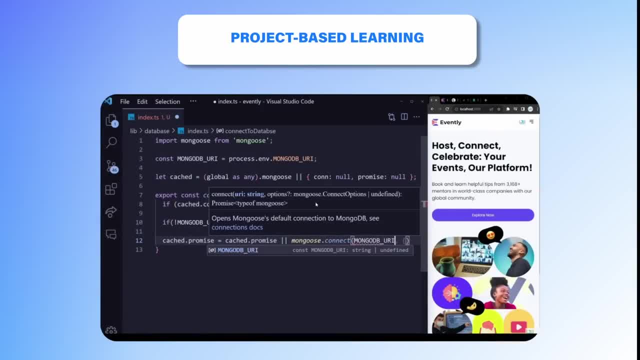 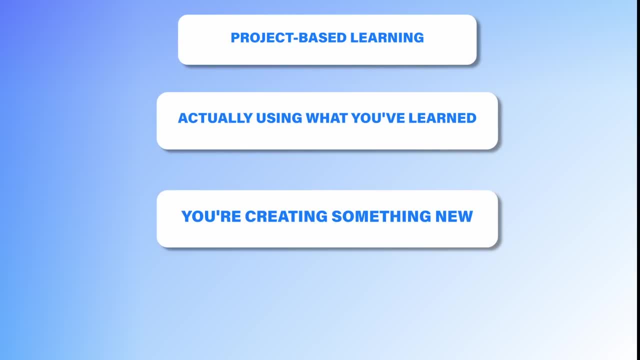 projects. You can still watch or read tutorials, like making a to-do list app, but the key difference is to add on to the tutorial and build other features from scratch. This way, you're not just following instructions, you're innovating and building your skills and. 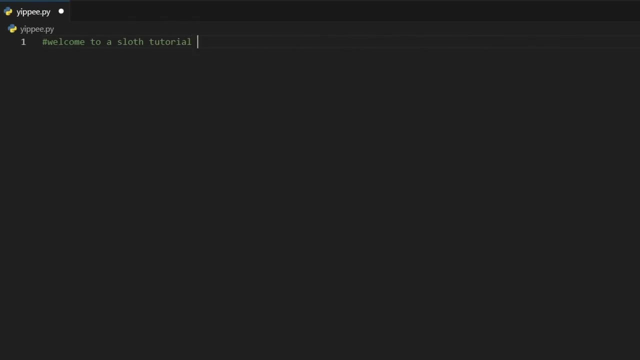 a practical, hands-on manner. For example, let's say you're watching a tutorial on making a calculator program. They show you how to add two numbers. Well, you can add on to the tutorial by adding a feature of subtracting two numbers. It wasn't in it, but you did it from scratch. 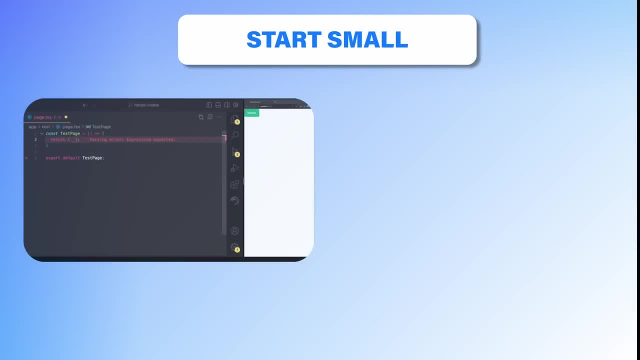 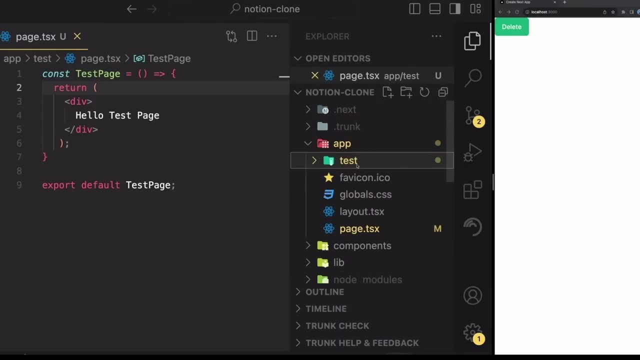 and now you're learning even better. Start with small projects. Maybe you want to build a personal website, or you know the simple calculator, And as you work on these projects, you'll encounter real problems and learn to solve them, which is a critical skill in coding. Not only does this